somebody. you know I'm smiling and I'm talking to them and I'm looking at them. I try to keep that connection, you know, really strong with them. You know I'm smiling and I'm talking to them and I'm talking to them, You know I'm smiling and I'm talking to them, You know. 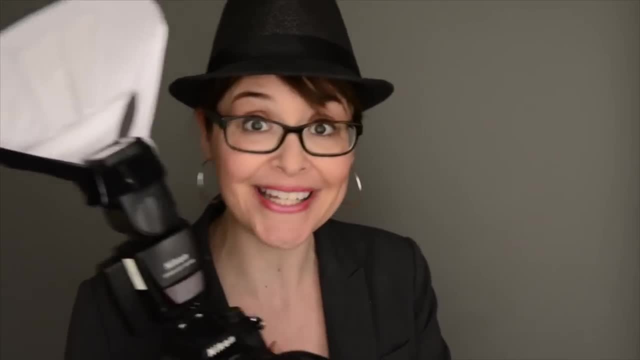 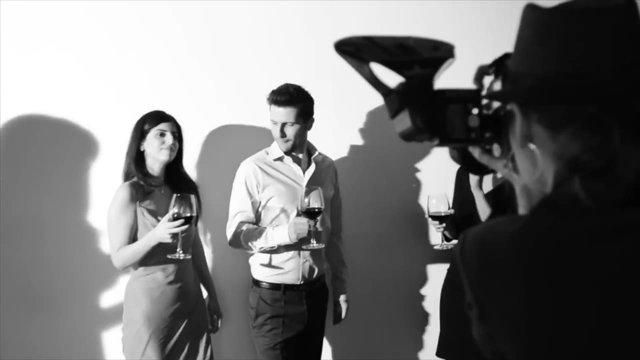 when you walk up to some group of people and you say, hey, would you like to get your picture taken, While they're arranging themselves, getting down their drinks, stopping chewing, putting down their plates, taking off their name tags, you can, in the meantime, be getting. 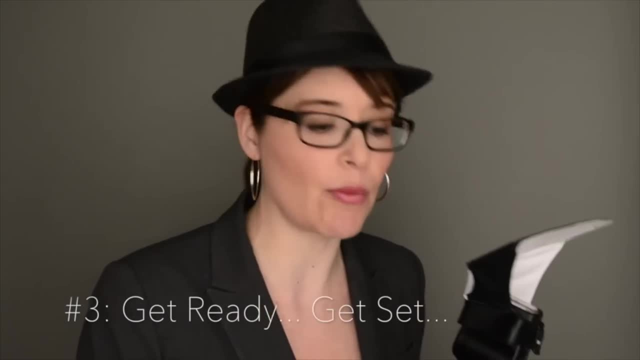 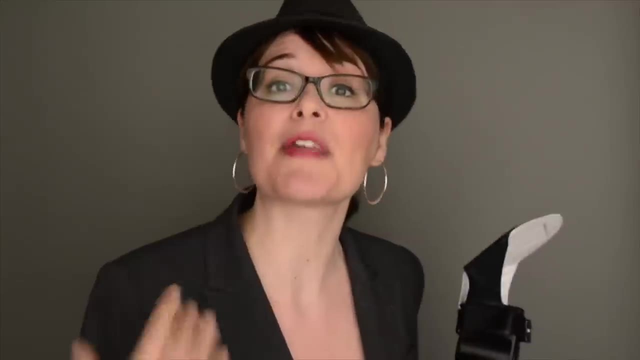 your focus ready, getting your composition straight. So that way, when they're like all ready to go and they're laughing and they're looking at me, they look at you and smile and you just go: hey, boom, boom, Keep things moving fast, so that way they don't have a 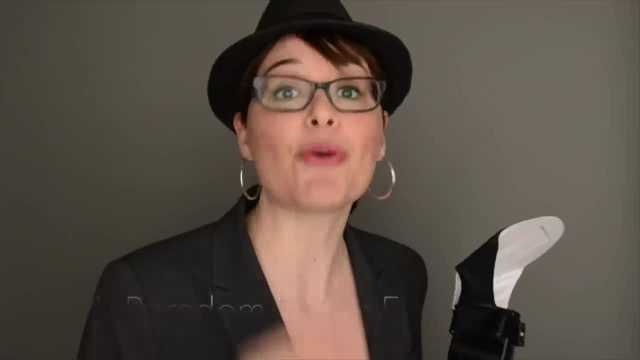 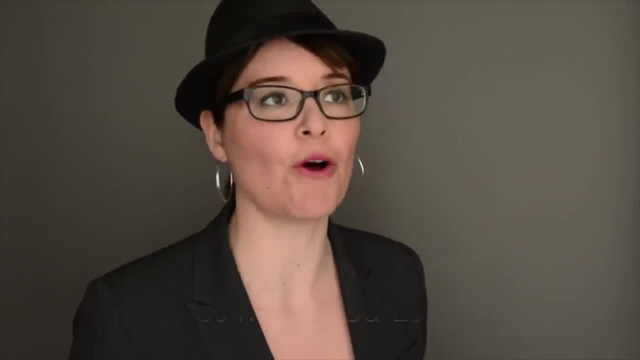 chance to get bored and kind of lose that smile in their eyes. So if you have that kind of connection with them and you're smiling at them and looking at them and you're fast, then you're more likely to get a shot where they're engaged- Yeah, people have like their 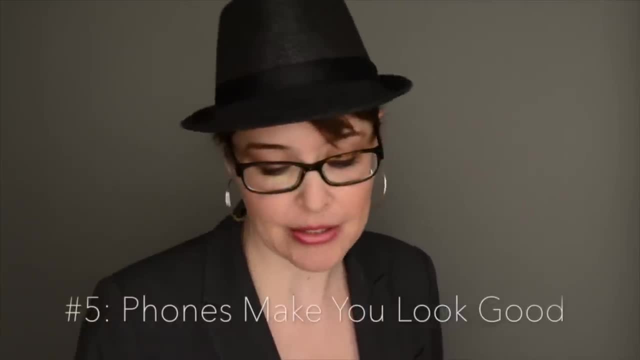 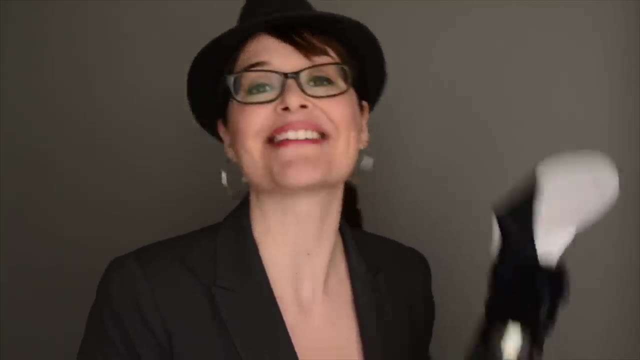 phones out and you can be so much faster than them, because, while they're kind of like hold on a second, hold on a second, you can be like this: You just go all right. all right, man, you're done, Awesome, thanks, Okay, great, Boom, boom, Because you're already set up. 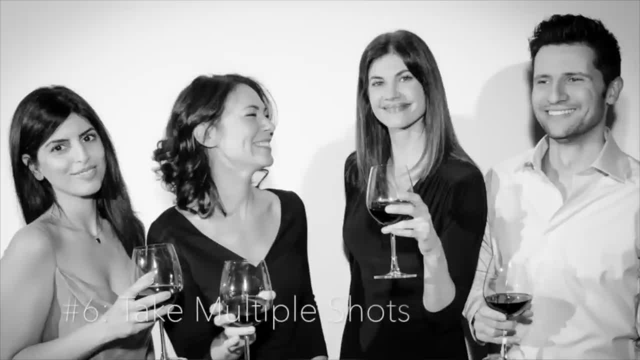 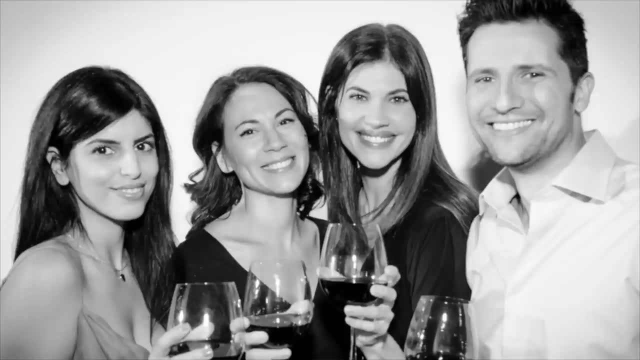 I take multiple shots. So if I'm photographing, let's say, two people, I take two pictures. If I'm photographing three people, I take maybe three pictures, Maybe five people, maybe about three pictures. It's probably fine. Something I really can't stand in: event photography is pictures of. 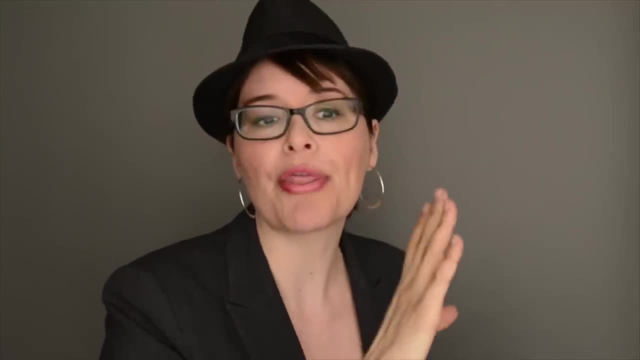 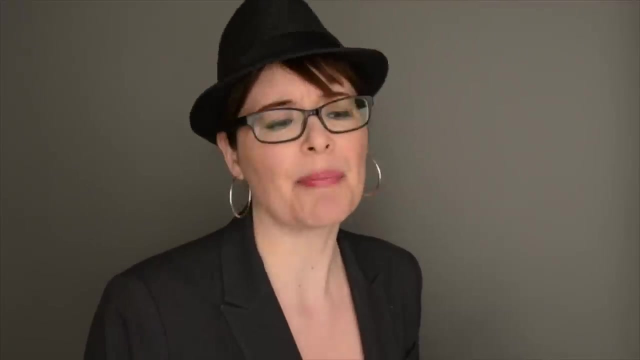 people right in the middle, framed exactly dead center, with all kinds of stuff around them that has nothing to do with them and what's going on and the fun thing that's happening at the event. A picture of some random thing, like as if there's like a fire extinguisher. 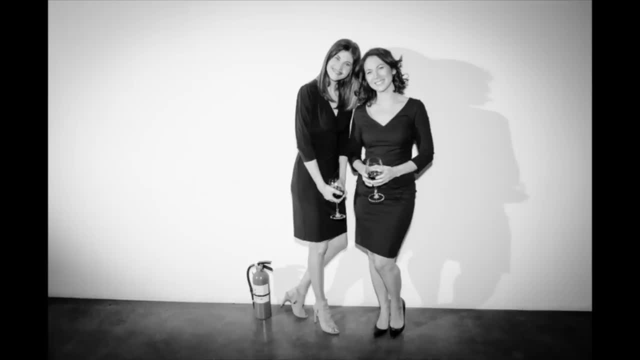 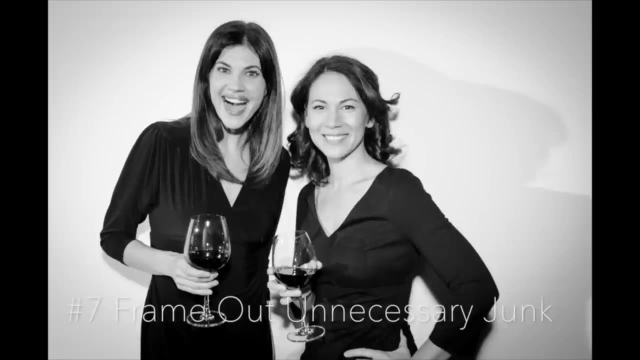 just sitting there and you're like, oh, I have to get the fire extinguisher in this shot. It's like, dude, why Frame it out? You know, zoom in step in This lens is a zoom lens, obviously, And zooming is very fast. 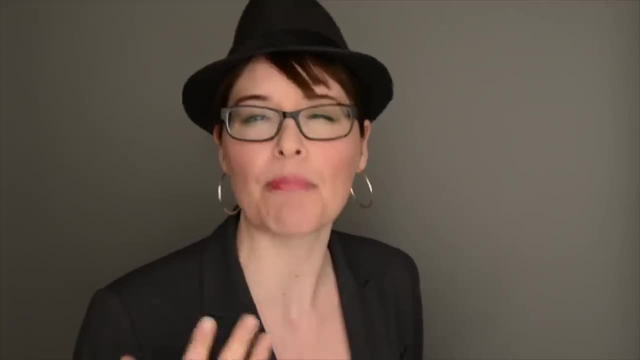 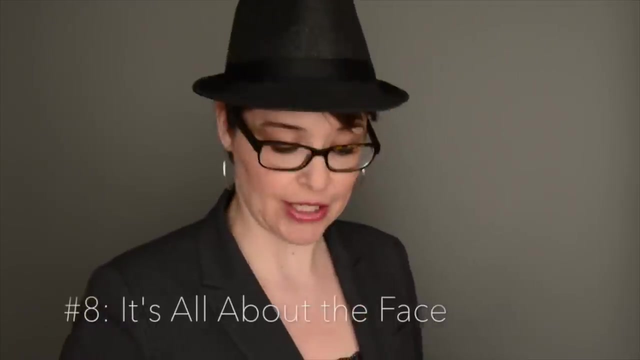 Fast and smooth. So just crop it out. you know, The most important part of the picture is their face. Make it all about the face. It is often more flattering to frame it from here up. anyway, Right, Let's say you walk up to a group of people and you're having trouble focusing because 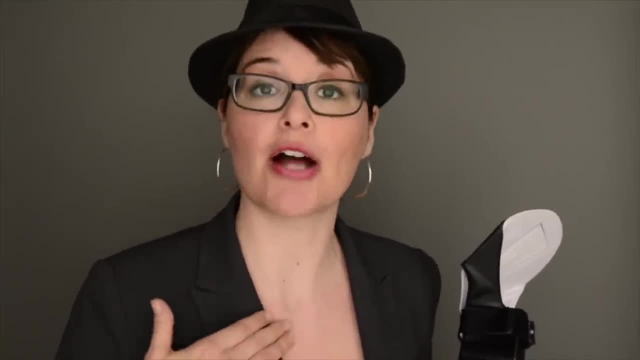 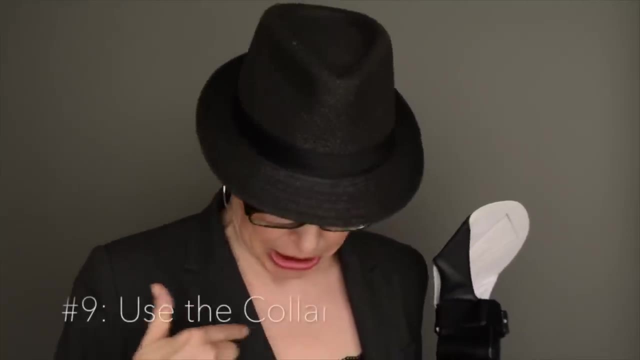 it's a little dark. It's a great tip to focus on an area of contrast that's on the same plane as eyeball, which is often like a collar. So you look at this, you know nice contrast. You can focus right here, Get a nice contrast.